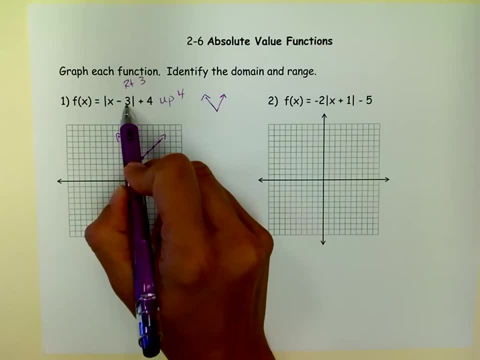 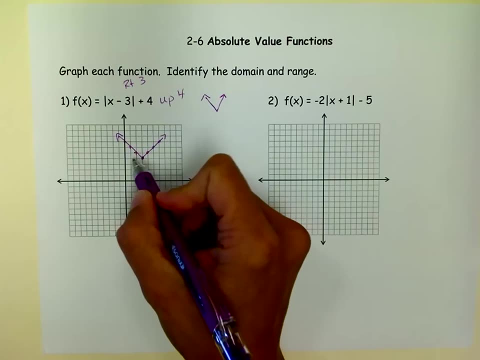 If I put a 2 in, 2 minus 3 is negative 1.. The absolute value of negative 1 is 1.. 1 plus 4 is 5.. So when I put a 2 in, I was up 5, which is what that says. 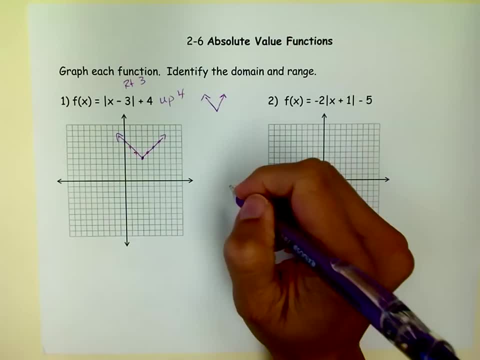 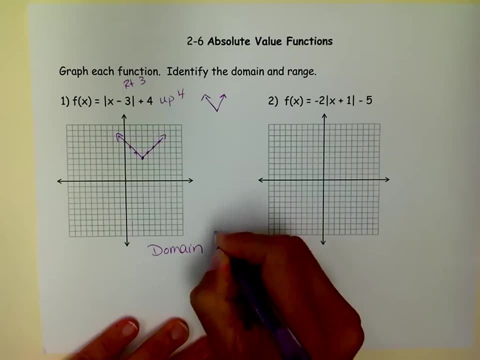 And you could make a little t-chart and do that. Well, now we need to figure out what our domain and range is. There's only two things. There's only two things that limit domain, And those are square roots with a variable in them and denominators with variables in them. 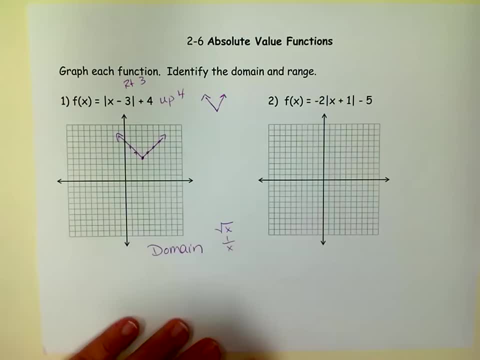 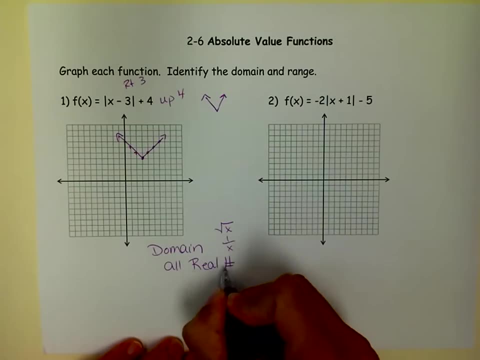 And you'll notice that these absolute values do not have either of those. So our domain will be all real numbers. There are different ways to write that. Some teachers are okay with all real numbers. Some teachers want you to use interval notation. So you would say negative infinity to positive infinity. 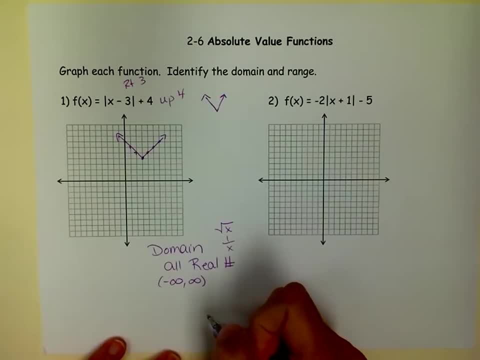 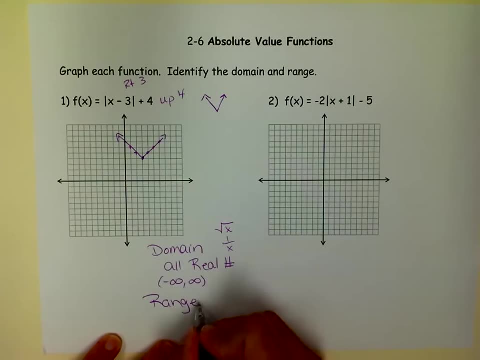 There's other ways to write it. You're just going to have to figure out what your teacher wants. The range now remember: the range deals with what y can be. Domain deals with what x can be For our range. we don't go down forever. 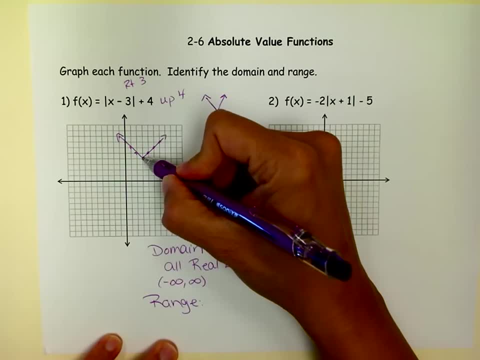 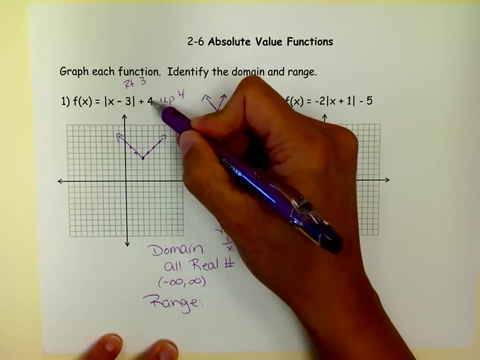 We just go up forever. So our range actually begins right here. So we need to find that y value And we went up 4.. And you can count that too. But this right here would tell you where your range would begin. So our range is anything bigger than or equal to 4.. 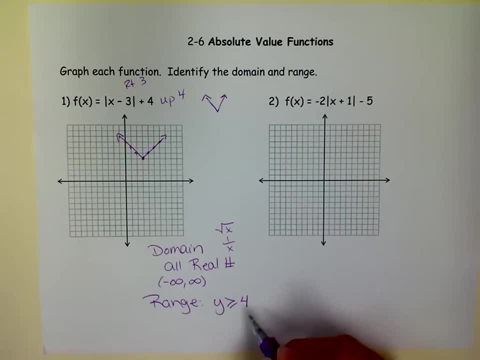 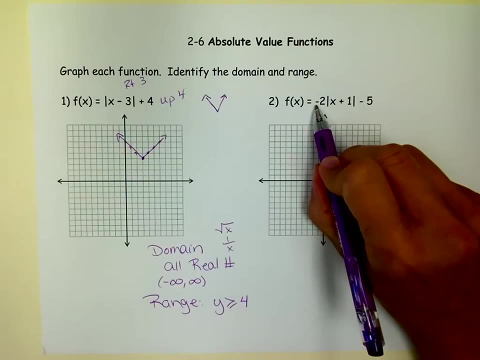 So we would say our range is: y is greater than or equal to 4.. All real numbers that are greater than or equal to 4.. Okay, let's look at this one. This negative sign tells me I'm flipped over the x-axis. 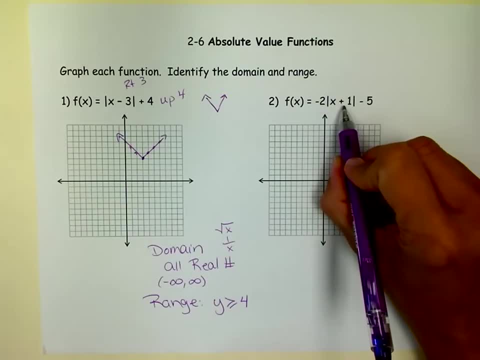 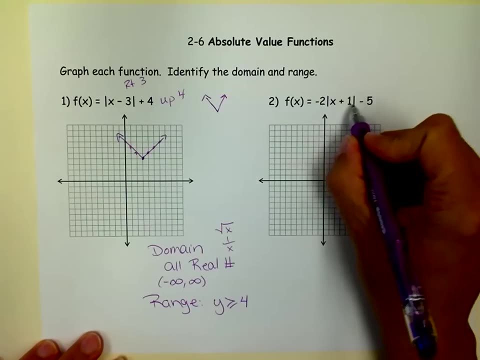 This 2 tells me I'm vertically stretched. This 1 tells me I moved left, 1. And this tells me I moved down 5.. So, keeping all that in mind, my vertex is now at negative 1, negative 5.. 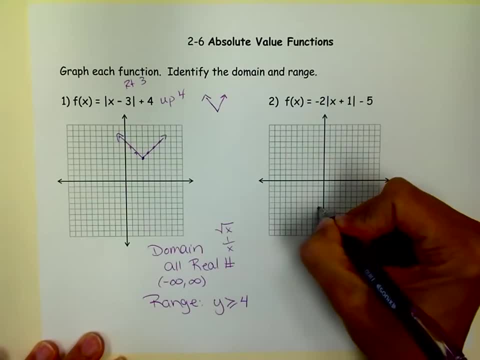 So negative: 1, 1,, 2,, 3,, 4, 5.. Now, normally on an absolute value function, you're going to be able to do this On an absolute value function like this one when it's not vertically stretched or shrunk. 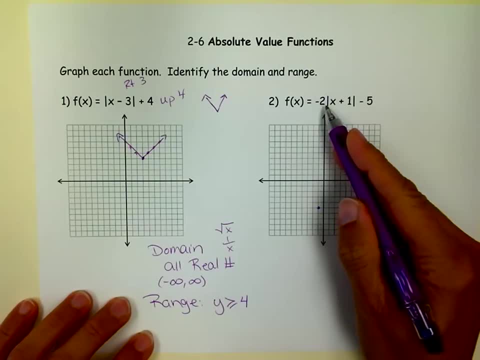 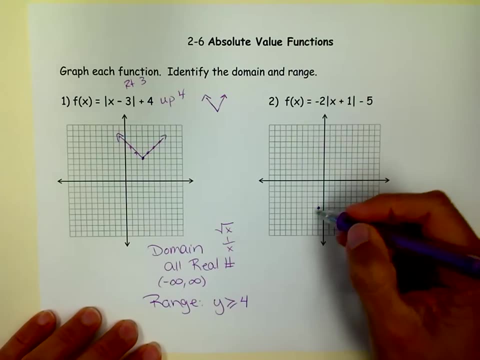 I would just go up 1 over 1.. Well, I can't now, Because now it's a factor of 2 on the up and down scale. So remember that. this tells you that it's upside down. This tells you it got skinnier. 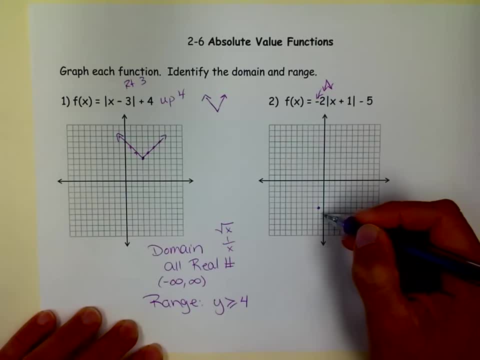 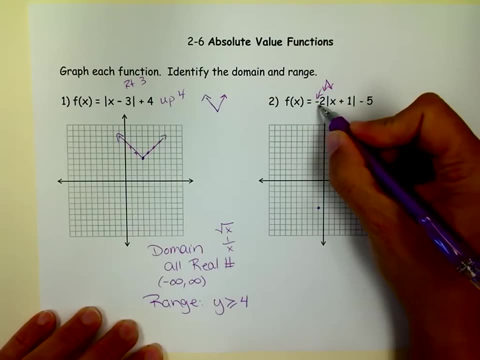 And this shifted it left and right, up and down. So if you're not sure, remember just put a number in: 0 plus 1 is 1.. The absolute value of 1 is 1.. Times negative. 2 is negative 2.. 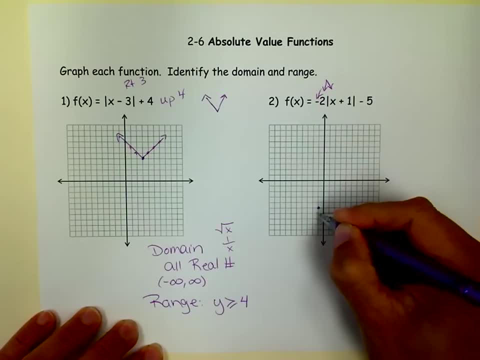 Minus 5 is negative 7.. So when I'm at 0, I'm down, negative 7.. So I want you to notice on the absolute value: traditionally, normally it would go up 1 over 1.. Look what happened. 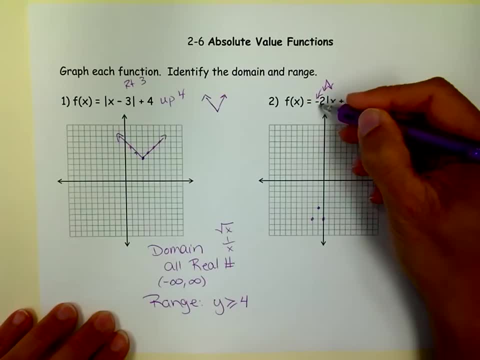 I went down 1 over 1.. Because of that 2. So this 2 kind of it's kind of like changing the slope on a line from 1 to 2, where you wouldn't go up 1 over 1,. 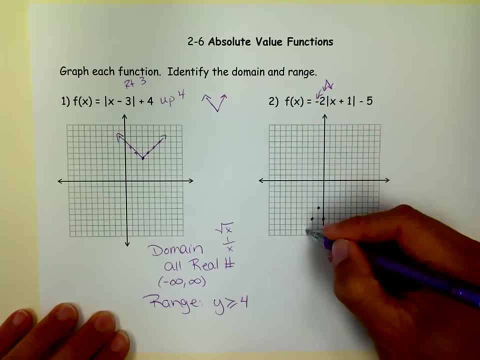 you'd go up 2 over 1. And so you can just keep that same pattern for this absolute value function, Because it's always going to be that 2, 1 ratio for absolute values. So now we need to find our domain. 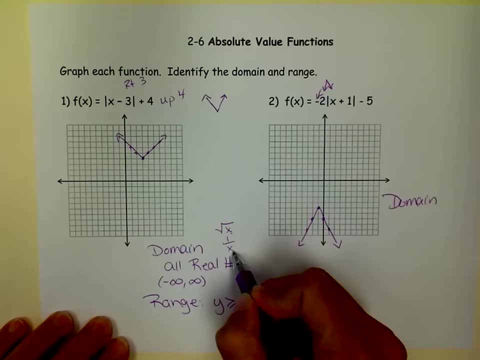 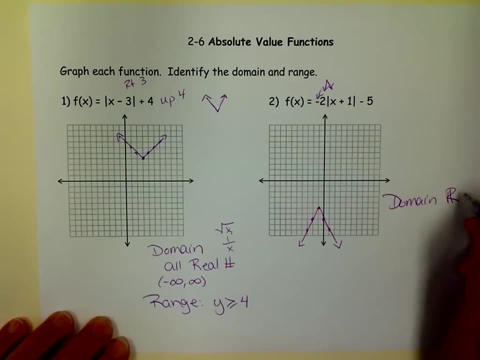 Our domain again: no square roots with x's, no radicals with- I mean denominators with x's. So our domain is all real numbers, And sometimes people use the real number symbol, The range. on the other hand, we don't go up forever. 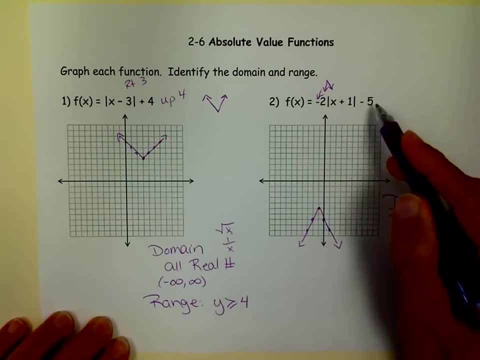 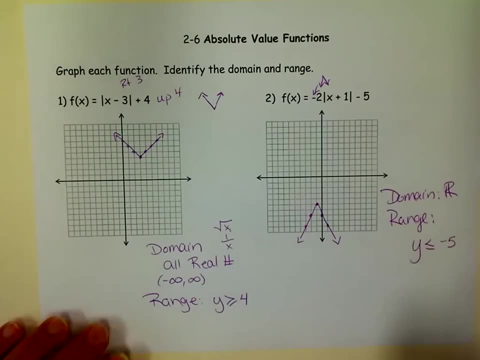 we go down forever. We started right here And our y value, since we were down 5, we start at negative 5.. So y is anything less than or equal to negative 5.. Good luck graphing absolute value functions. This is m squared sine of.